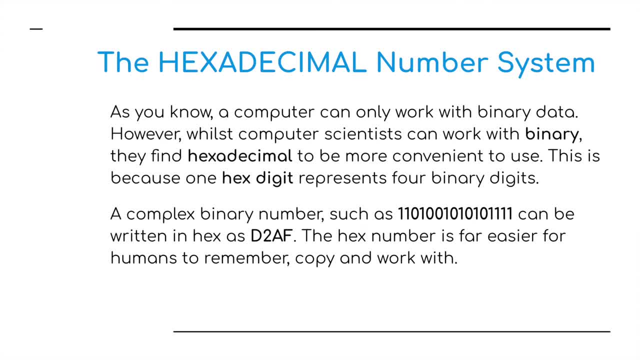 work with binary digits. The digits represent the transistors on the CPU and whether they're in an on or an off state. Computer scientists can work with binary, but they find hexadecimal a more convenient thing to use. This is because one X digit represents four binary digits, so something really long like the number. 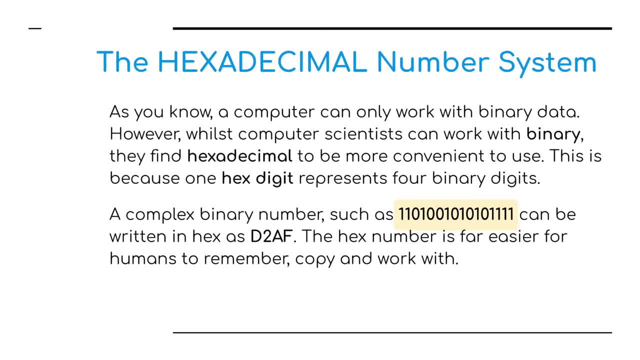 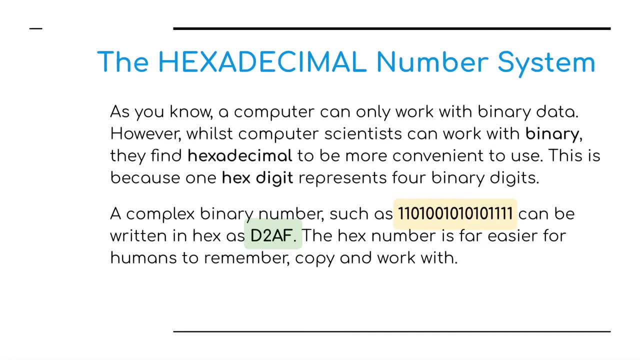 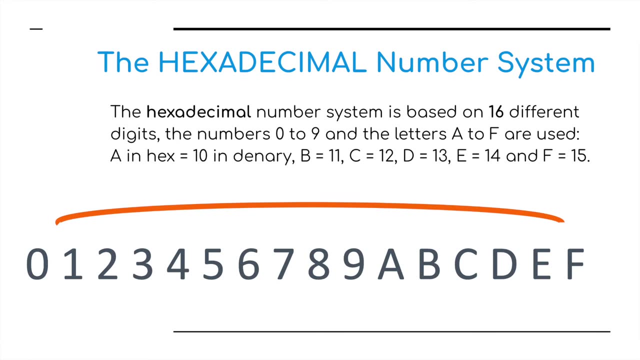 below this number here can be represented, and the 16 bits can be represented as four different digits, in this case D to AF. It's easier for a person to remember. Before we begin, let's have a little look at what exactly is the hexadecimal number system. 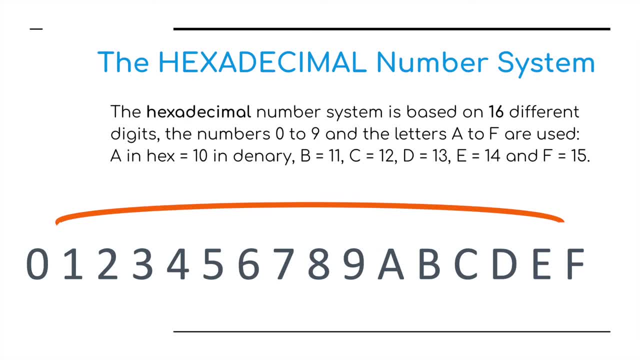 It is a number system based on 16 different digits. The same digits as they are in base: 10, 0 to 9, but because of 16 different digits or characters, we also include A for representing 10,, B, 11,, C, 12,, D, 13,, E, 14 and F 15.. In base 16 we're. 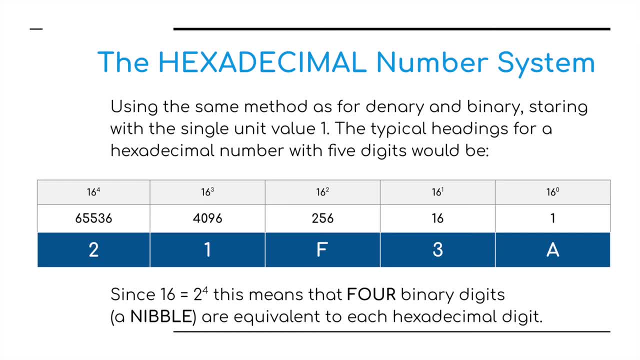 going to start with the units column and then, when we get to 16, times it by 16 times it by 16.. So we have 1, 16, times 16 is 256, times 16 is 4096, and so on and so forth. 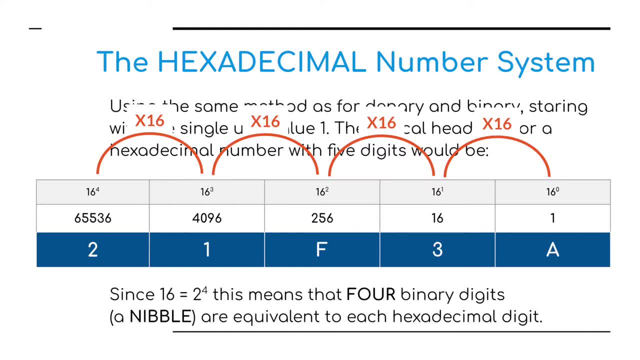 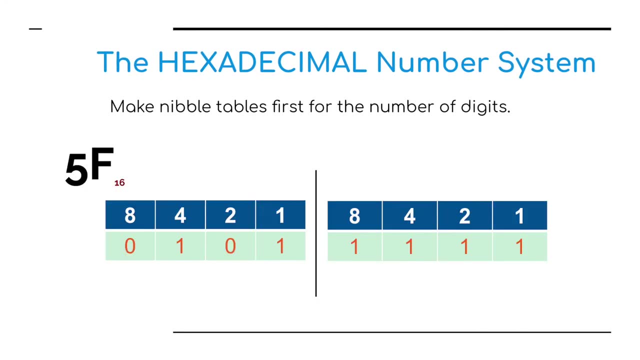 Now, since 16 is 2 to the 4, this means that there are four binary digits- or a nibble, as we've covered before- that are equivalent to only one hexadecimal digit. Well, what does that mean? Well, if we look here, we have a two digit hexadecimal. 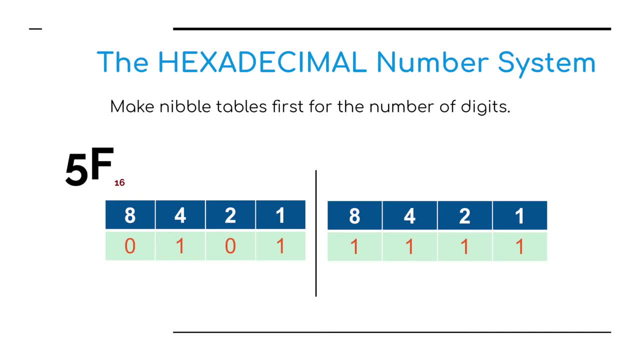 number 5F. Now we can break those two numbers down into into two nibbles. For example, as you can see there we've got the nibble on the left representing the 5 has a value of 4 and 1.. 4 plus 1 is 5, and on the other side, on the right hand, 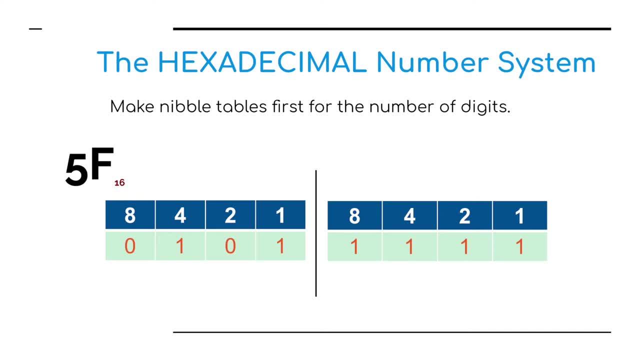 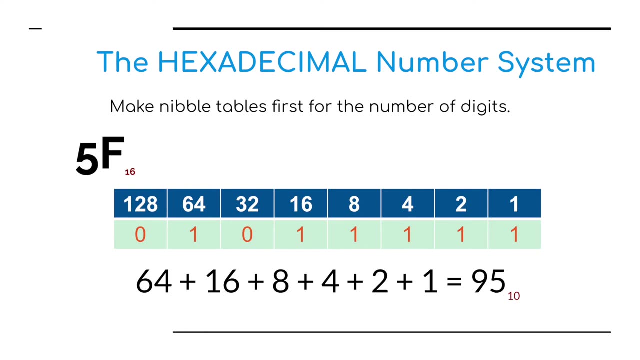 column, we've got F, which is represented by 8 plus 4, plus 2 plus 1, which is 15.. So 5F equals 0, 1 0, 1 1 1 1 1 in binary. To take that step further, if we forget about the two nibbles for the time being, 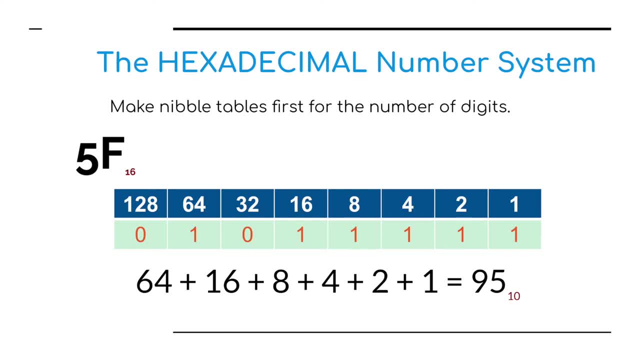 and go back to the old system that we know- 1,, 2,, 4,, 8 and then doubling every time up to 1,, 2,, 8 or a byte of information- we can see that we've got one lot of 64, a 16, an 8, a 4, a 2 and a 1 and we add all those numbers together and we 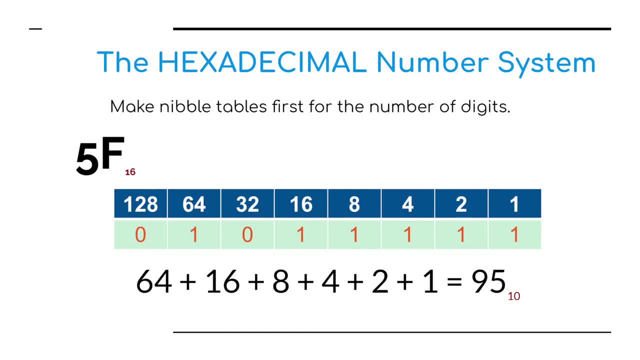 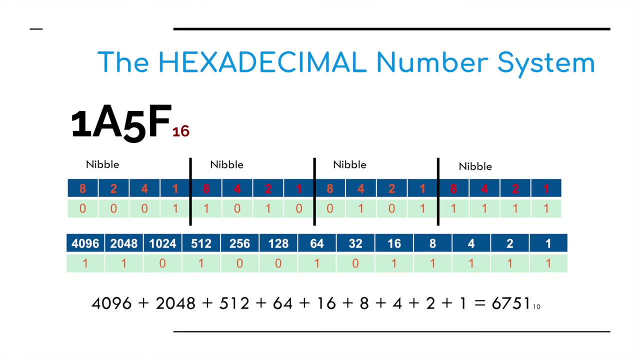 have a base 10 number, a decimal number of 95. We can take this a stage further. we'll look at a bigger number now, 1A5F, So that would be, F would be the unit, so 15, lots of 1s. 5 would be the 16. 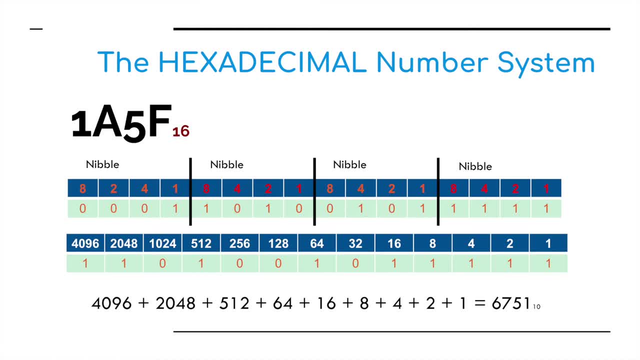 column, so 16 lots, sorry, 5 lots of 16, A would be the 256 column, so 10 lots of 256, and 1 would be the 4096 column, so 1 lot of 4096.. So let's break. 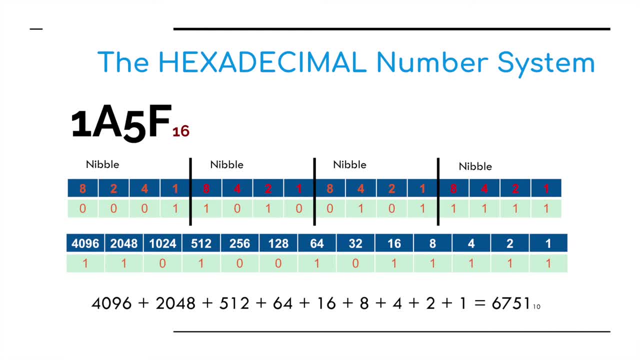 that number down into four. We've got four parts, a nibble for each of the numbers in the. in those four digits We've got a 1 in the. in the first nibble we've got 10 or A. for the second nibble, 5, 4 plus 1 for the third nibble, and then 1, 1, 1, 1 or 15, which? 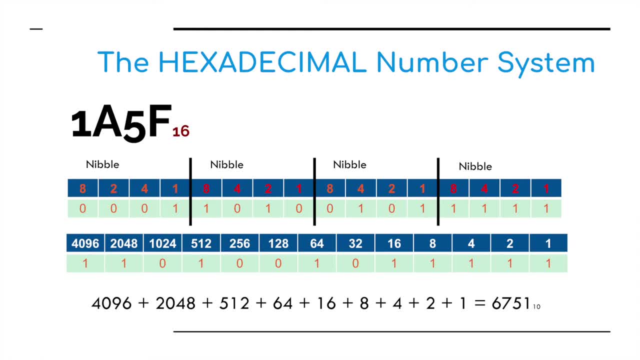 would be F for the, for the last digit. Remove the lines, remove the nibbles. we can see there we have a number adding all the 4,096 plus 2,048.. Add them all together where the 1s are, we have a. 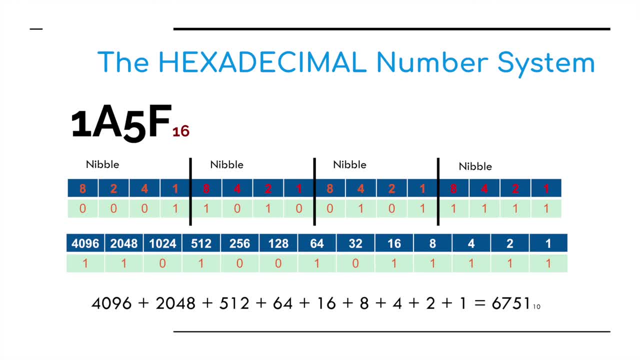 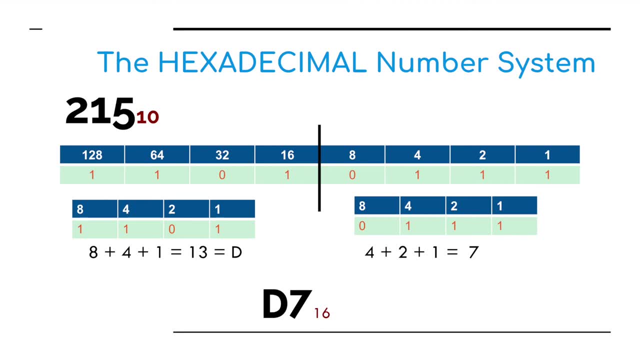 number, a decimal number of 6,751.. We can go the other way. If we start with a base 10 number, I'm going to convert this into binary. So, as you can see there, one lot of 1,, 2,, 8,, a 64,, a 16,, a 4, 2 and a 1 would all add up to 215, 215.. I put the line back in to: 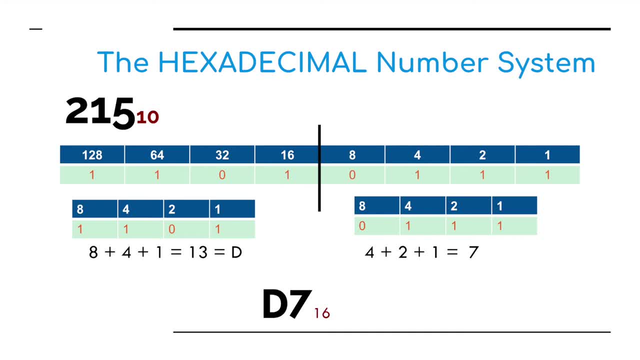 split it into two nibbles. So the left hand column: we have 8 plus 4 plus 1, which would equal 13, which we know is D in x-decimal, and with them we have a 4, a 2 and a 1 on the other side, which equals 7.. So 215 in base 10 converted to: 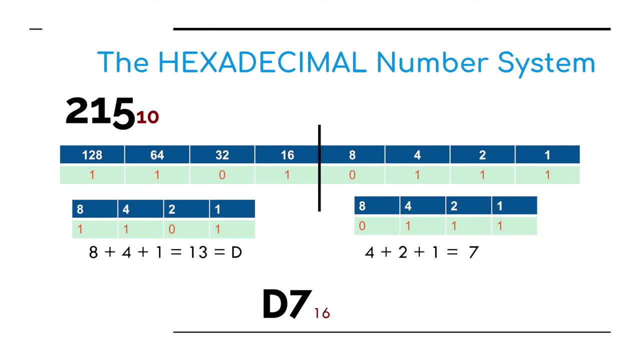 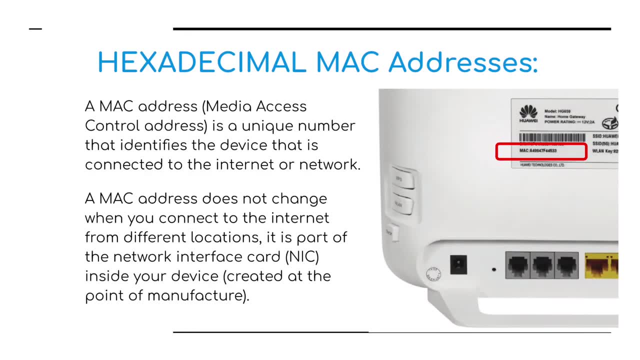 x-decimal would be D7.. What do we use x-decimal for? Well, let's start with MAC addresses Now. MAC address, or a media access control address, is a unique number that identifies a particular device that is connected to the internet or the network. 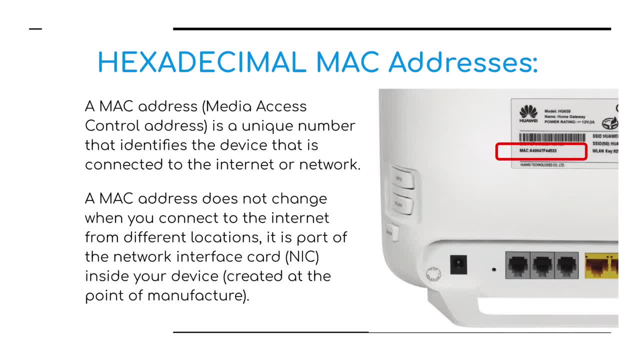 Any device. it could be Apple TV, it could be your, your MacBook, a computer, anything at all that's connected to the internet. We've got here a picture of a Huawei, a router in your house that's connected, that you connect to in order to 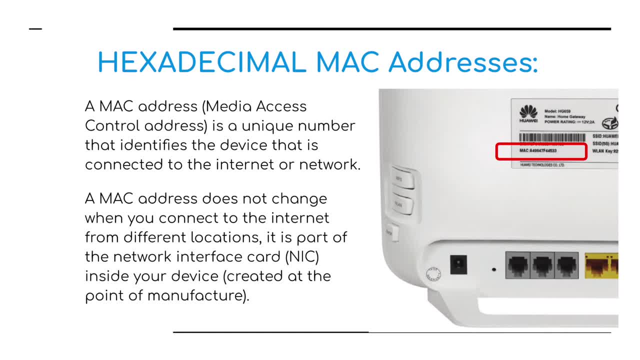 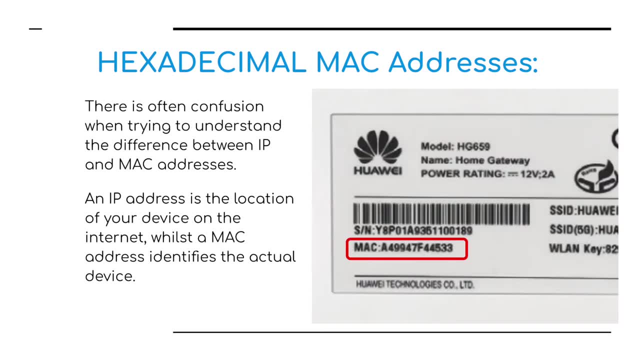 get onto the internet. The MAC address doesn't change when you connect to the internet. It is unique to that particular device. So in your computer you have a network card, a NIC card, and on that card, or part of that card, is its unique identity. 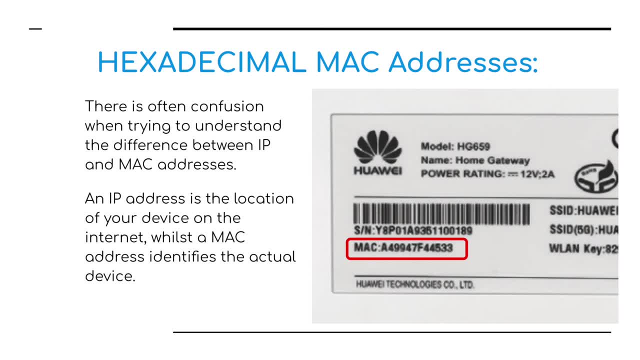 Thank you. There's an example of it here. There's often some confusion between MAC addresses and IP addresses. An IP address is the location of your device where it is on the Internet, whereas the MAC address is actually what the product, what the thing is that is connecting to the Internet. 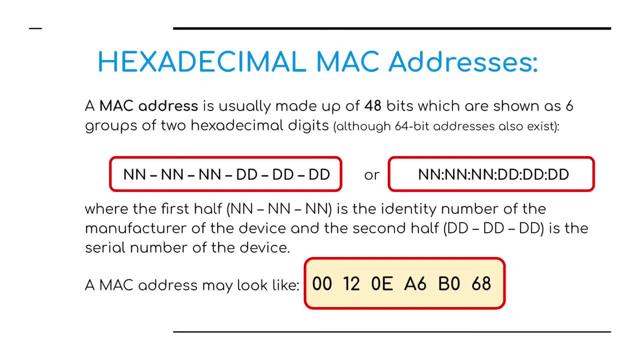 You can see some examples of 48-bit MAC addresses here and you can see it's broken down into two parts. The first part, the NNNNN, refers to the manufacturer, be that Apple, be it Cisco, Dell or whoever. 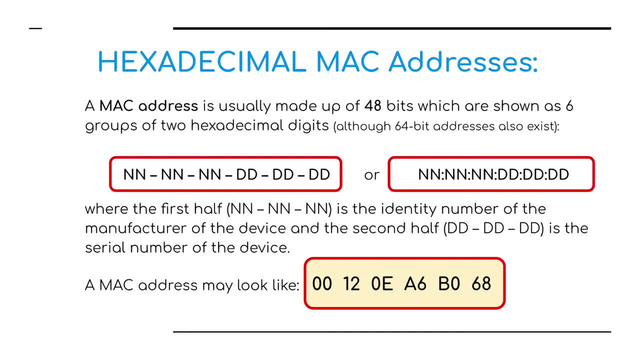 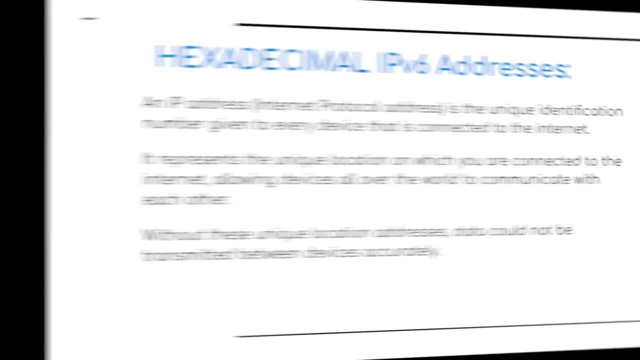 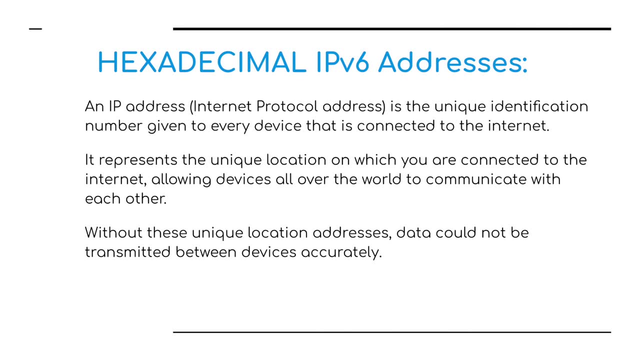 The second six characters refer to the actual serial number, the unique serial number of the product. There's an example at the bottom. Next is the IP address, the Internet Protocol Address. This is a unique identification number Every device has that is connected to the Internet. so this is where the confusion might. 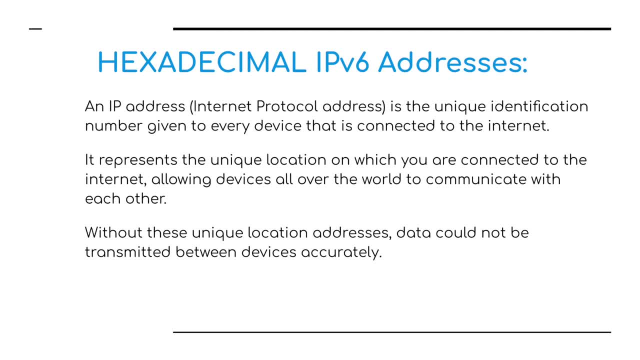 lie in terms of this and the MAC address. It represents the unique location on which you are connected to the Internet, allowing devices all over the world to communicate with each other. It works a little bit like a postal address. If the post office has some letters to deliver to you, they need to know where you live. 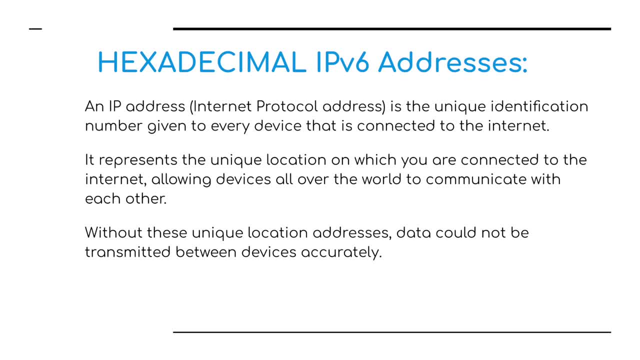 This is exactly the same for the Internet. The Internet needs to know where you are In order for you to receive e-mails and for devices to communicate with each other. When you connect to the Internet, you are assigned an IP address to use for your particular. 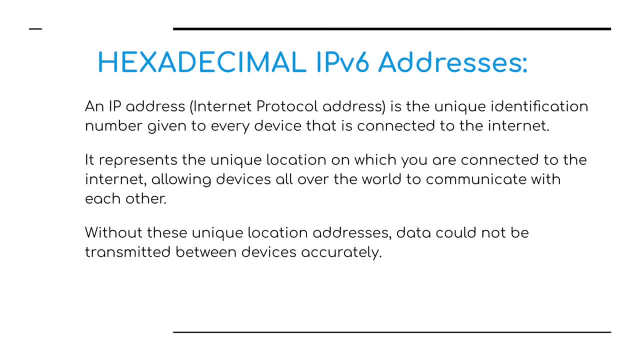 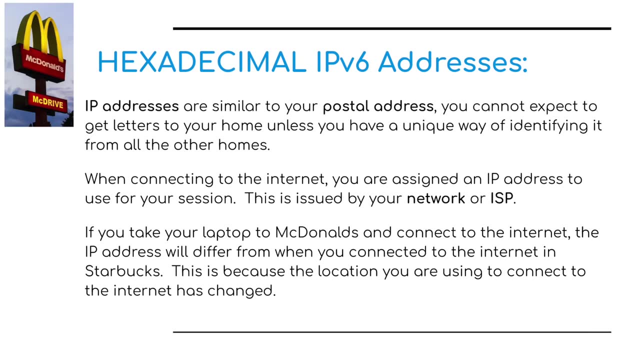 session. This is issued by your network or your ISP, something like Vodafone or Iliad or whoever you use for your Internet Service Provider. To give you a real world example, If you were to take your laptop to McDonalds and connect to the Internet, then your device. 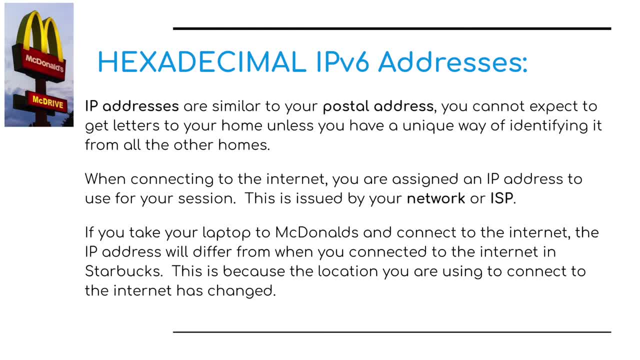 would be given an IP address If you decided that after you'd had your McDonalds and you wanted to have a coffee, but you didn't like the coffee at McDonalds, you wanted to go to Starbucks. So if you got up and walked to Starbucks, um, and then connect to the Internet there, 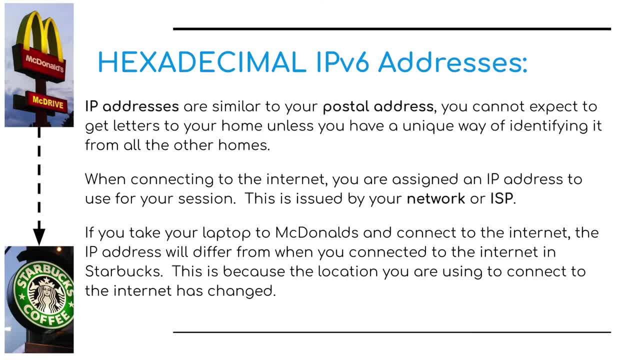 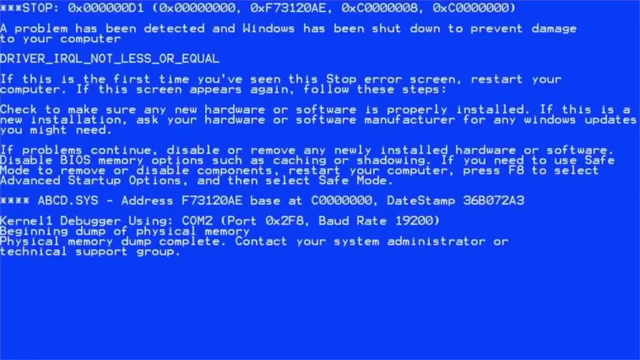 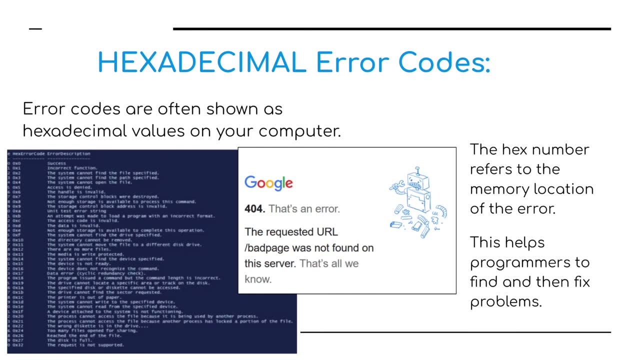 then you would be assigned- or your device would be assigned- a different IP address. If we move on to error codes, error codes is a very short part of this. Error codes are often shown as x-decimal values. Windows uses them a lot and you may be familiar with. 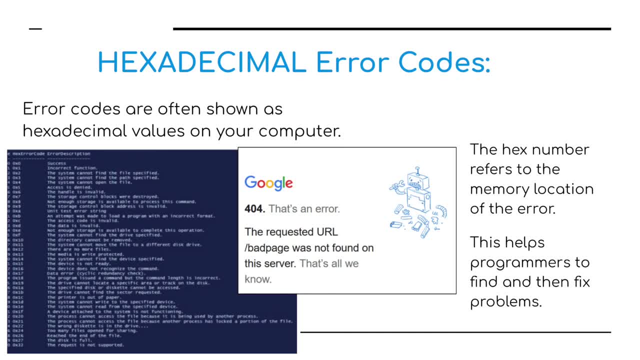 404, page not found various things. But they're also used for things like printers, even washing machines, devices that have a microcontroller, that may have a little screen and if something goes wrong then an error message might pop up. It's great for people service engineers. 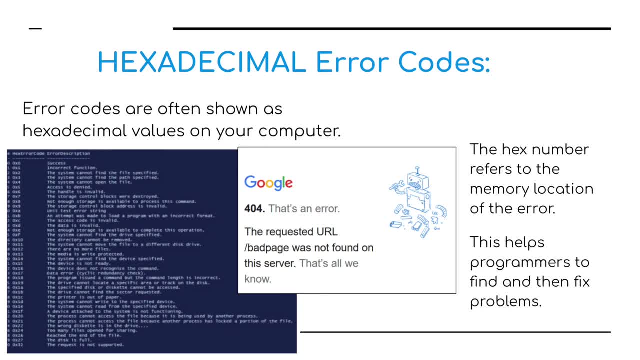 if they need to fix a problem, they can see the little error message and they know what the problem is. For example, with a printer, if you get a certain message, it might just mean that there's a paper jam or it might mean that the printer is out of touch. 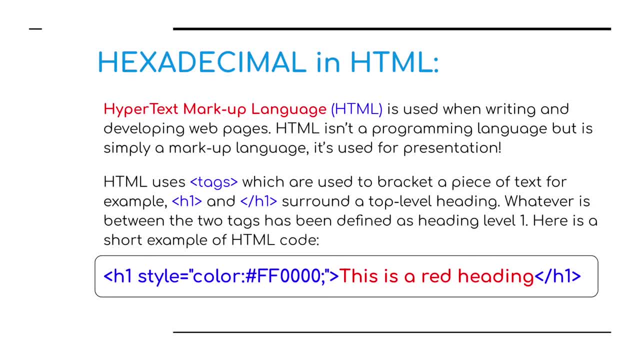 Finally, we need to look at how colour is represented using x-decimal. for websites, for webpages. So HTML hypertext markup language is used when writing and developing webpages. It's a markup language rather than a programming language, and it's used for the presentation.